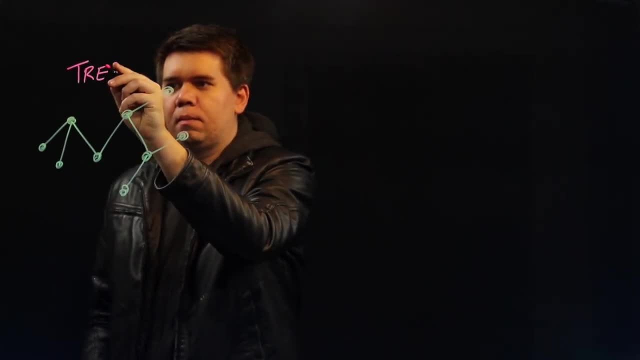 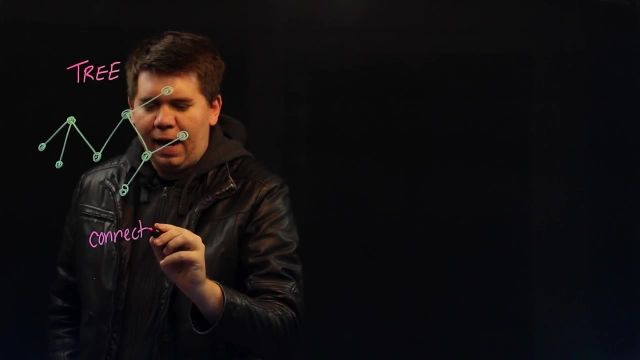 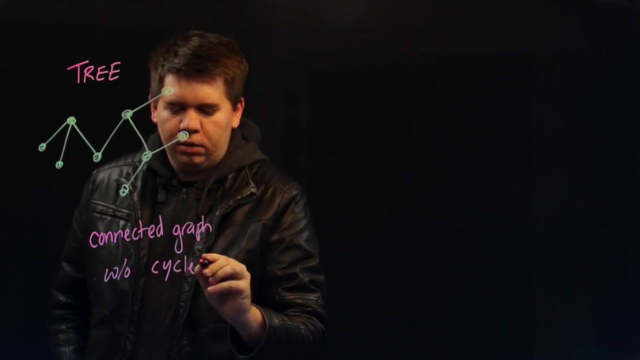 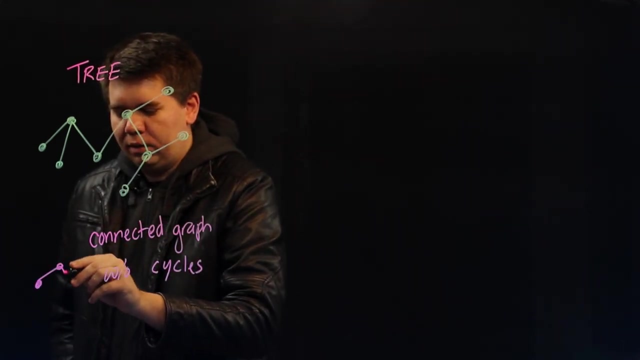 Here we have a tree. One way to define a tree is: a tree is just a connected graph without any cycles We call a cycle is just a collection of distinct edges and vertices that come together so that the first vertex is also the last vertex. 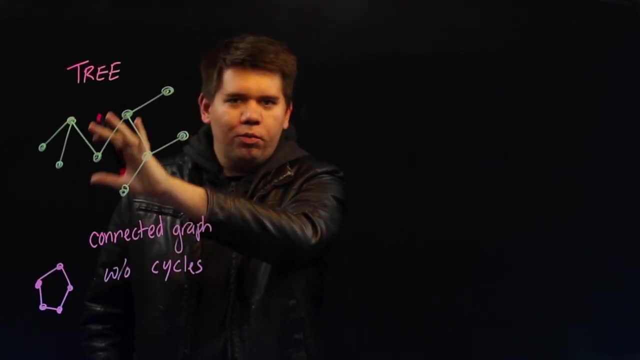 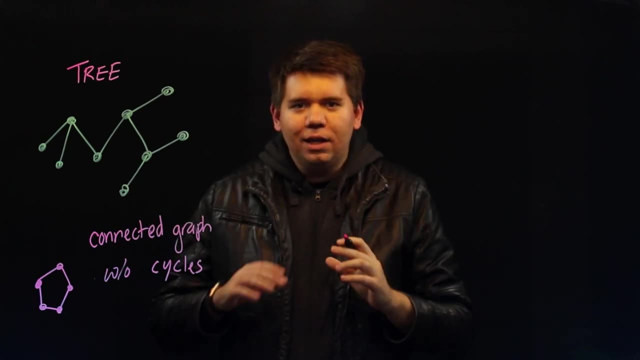 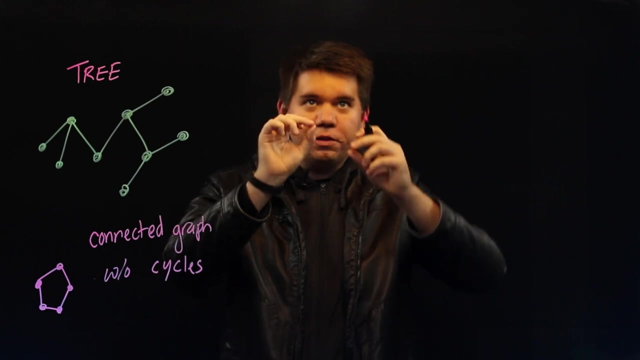 It closes into a cycle In a tree. we have no cycles Now. trees are important because we often store data in trees. For example, you can think of your family tree. Well, you have a parent and their offspring, and that parent is the offspring of some ancestor. 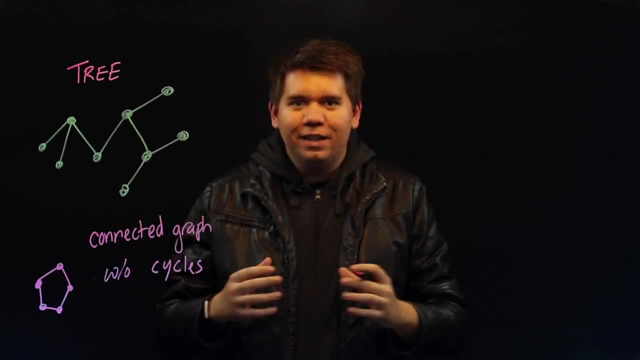 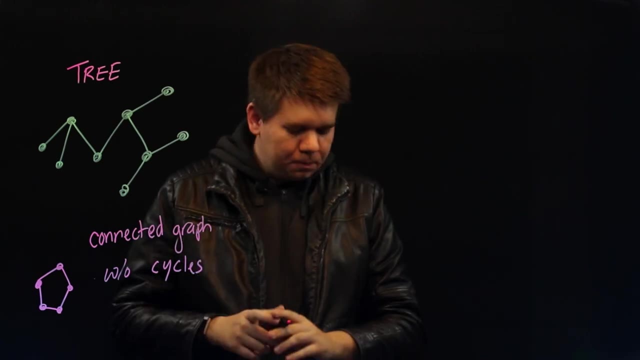 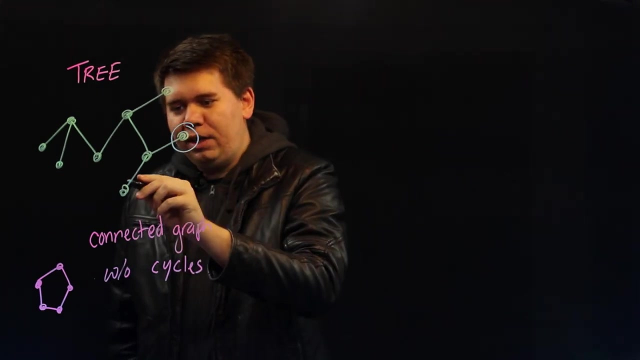 You can go back and represent your family data in that- family data In the form of a tree. What we're interested in are what are some of the properties of trees? You might notice that on a tree there are many leaves. That is, on a tree you will have vertices. 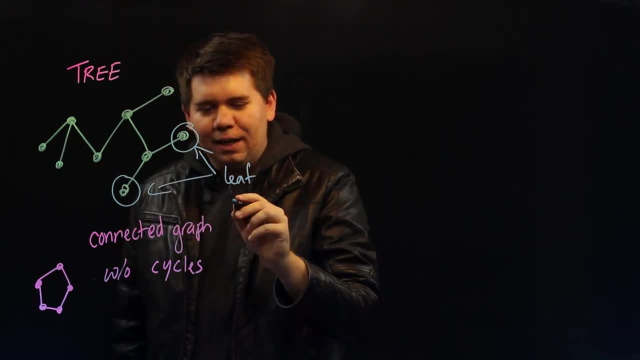 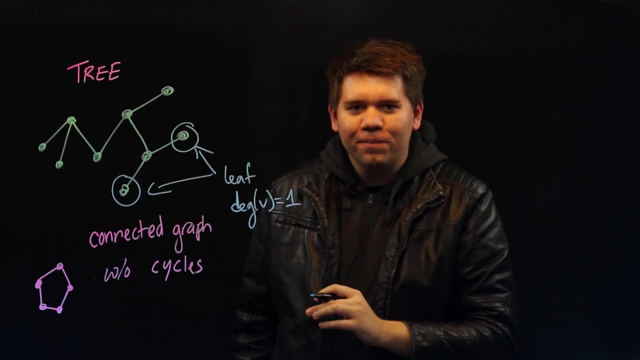 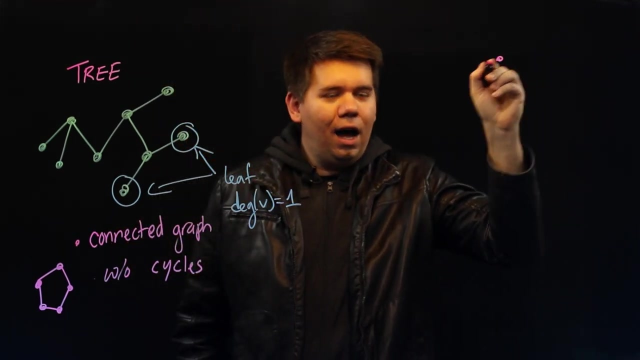 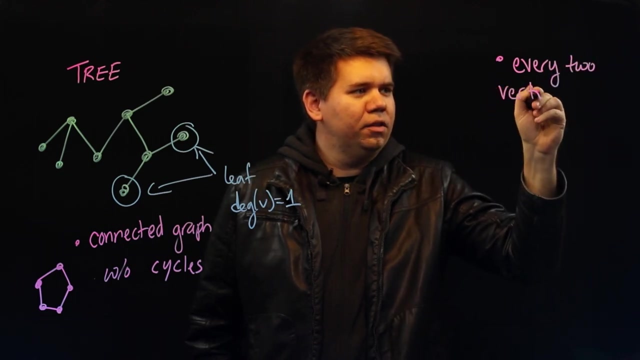 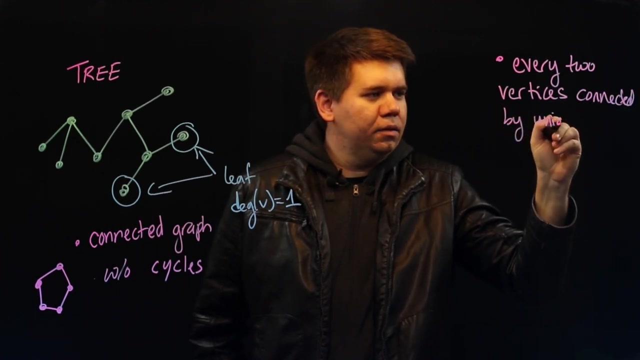 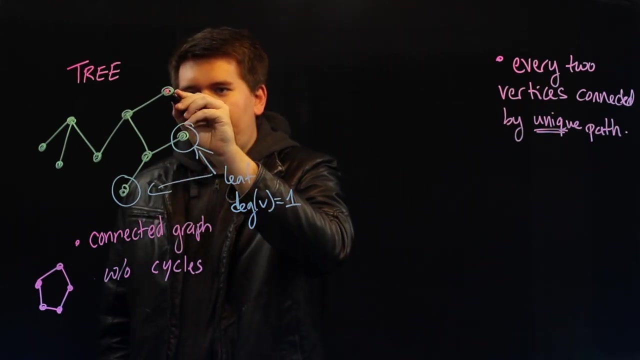 that have degree exactly one. We call these the leaves of the tree. What else can we say about trees? Another important property of trees is that on a tree, any two vertices are connected by a unique path. For instance, if I pick these two vertices, 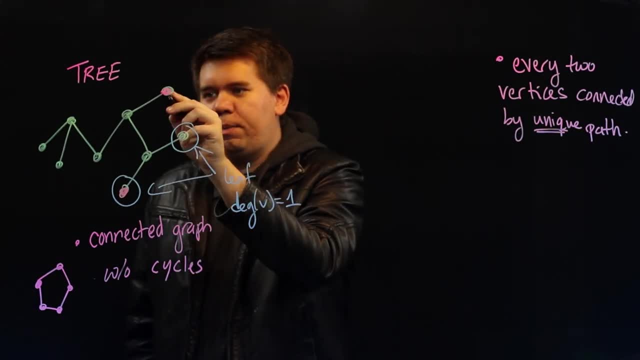 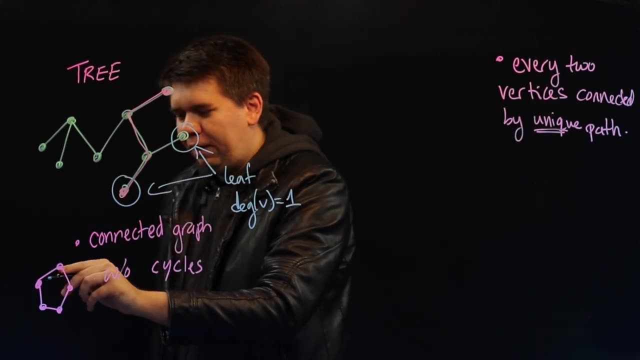 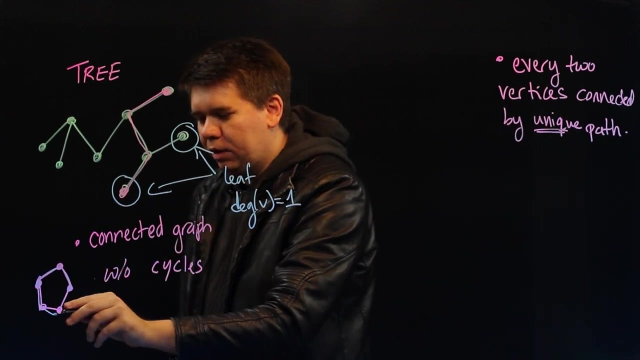 there is exactly one path That will take me from the one to the other. This is not the case in a cycle. In a cycle, if you pick two vertices, you have two paths. You can either go above or you could have gone below. 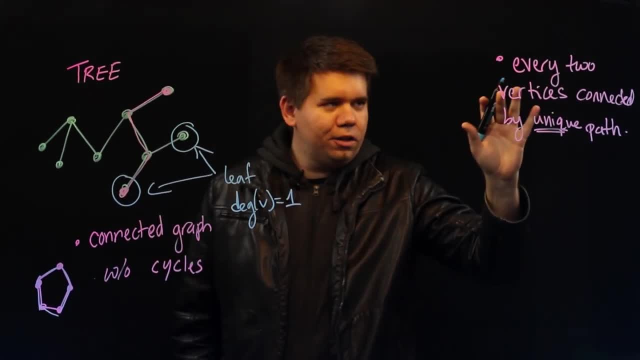 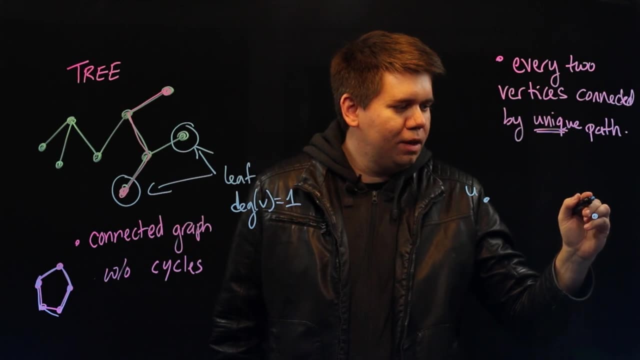 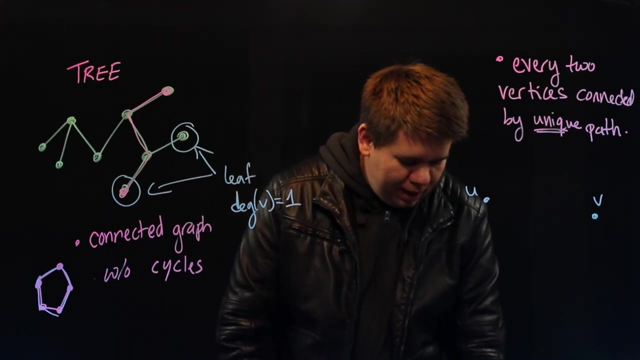 And in fact that observation is exactly the justification for this property. So if you had two vertices, call them U and V, inside of some tree that were connected by a unique path, that were connected by more than one path, then we can think. 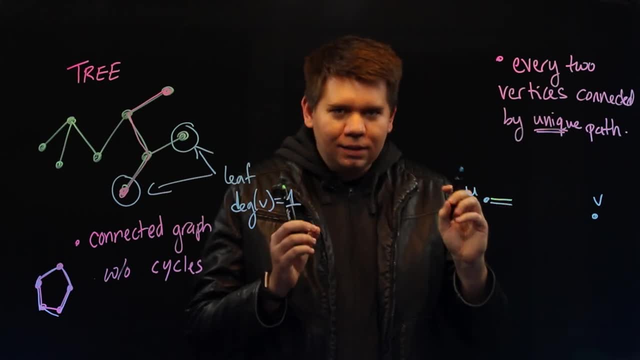 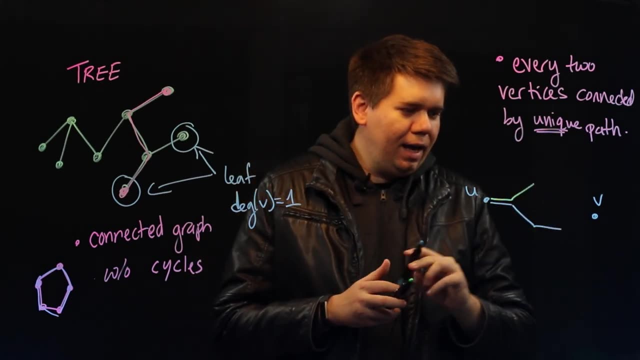 For a while, those two paths may be the same, but if they're distinct paths, then at some point they'll have to diverge from each other. And yet, since they're going to end up at the same place, at some point, those paths are going to have to. 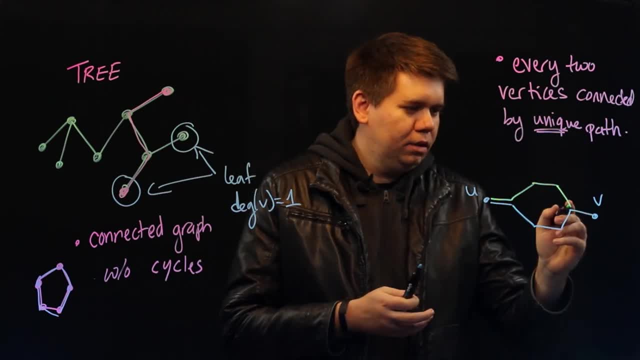 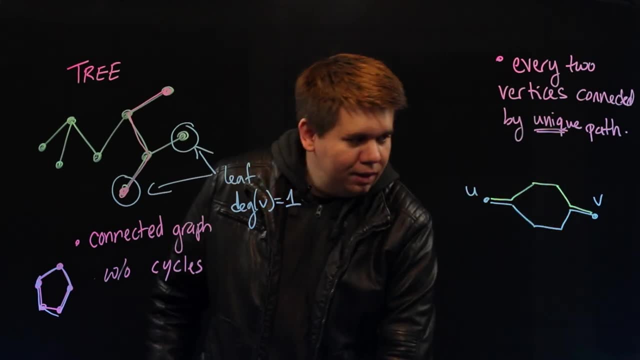 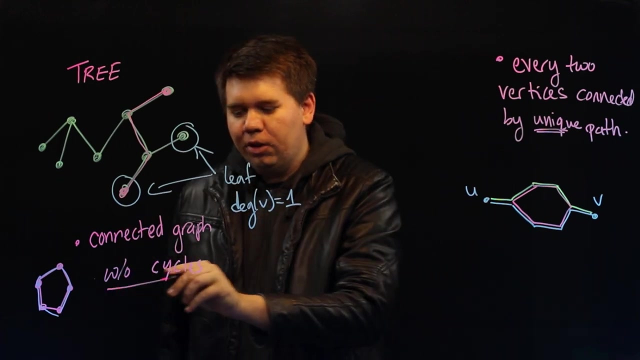 converge again and meet. Why can't this happen in a tree? Well, if you did have these two distinct paths between U and V, then notice they will form a cycle in your tree, And we define a tree to be a graph without cycles. 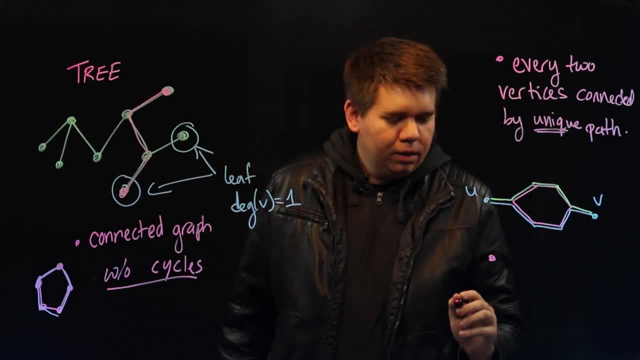 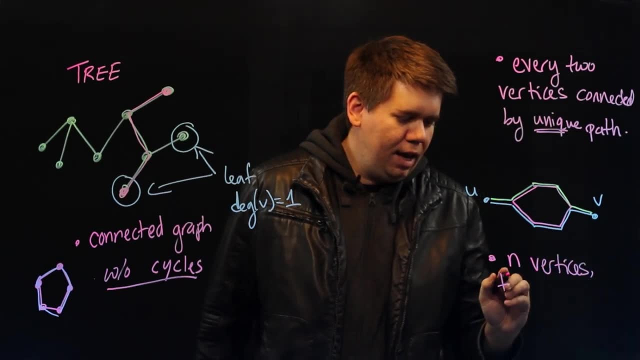 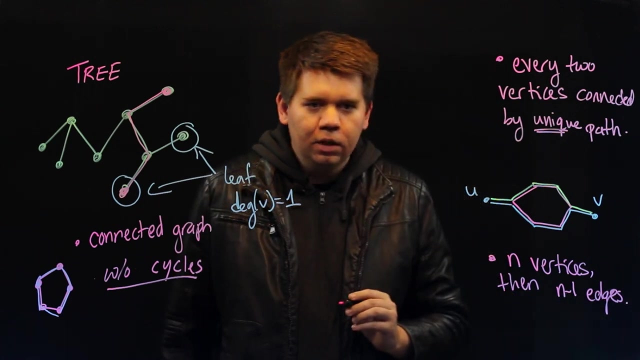 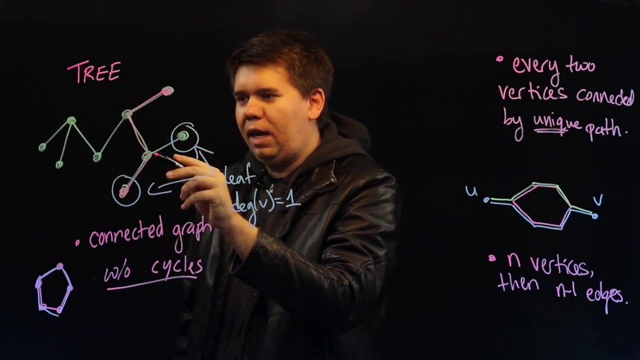 There's another property: of trees. If your tree has N vertices, then it has N minus one edges. So we might check this really quick. In this particular tree there are one, two, three, four, five, six, seven, eight, nine vertices. 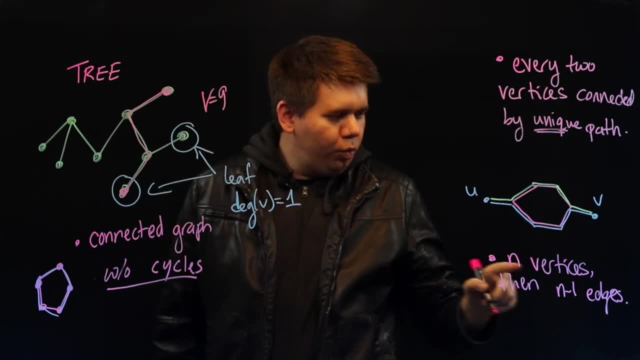 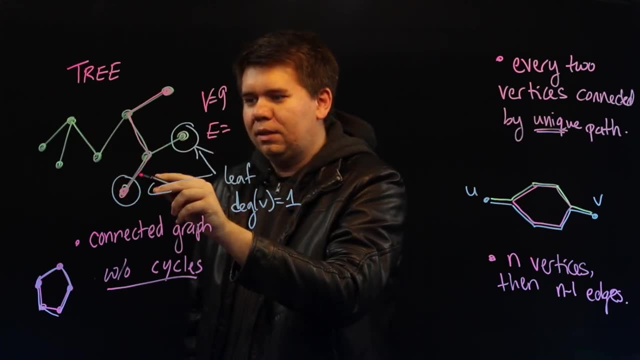 Our number of vertices is nine, So we should expect there to be eight edges. And let's check: There's one, two, three, four, five, six, seven, eight, Eight edges. Why is this true in general for trees? 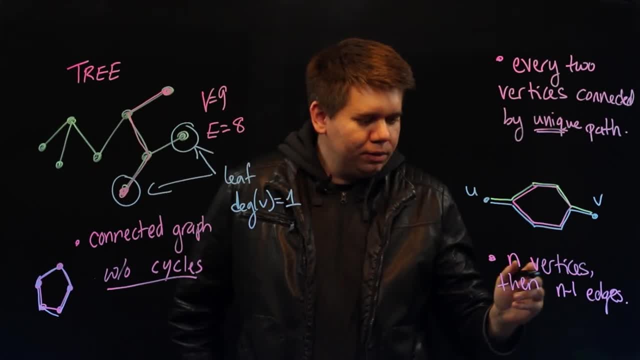 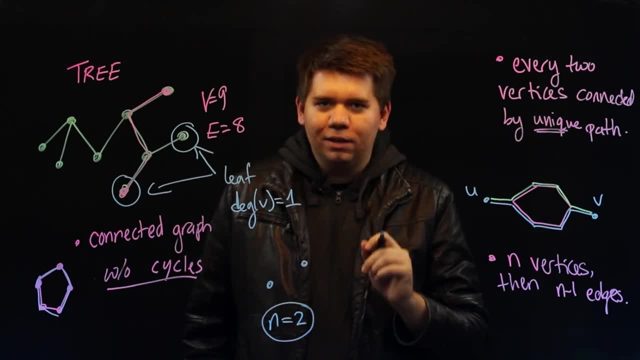 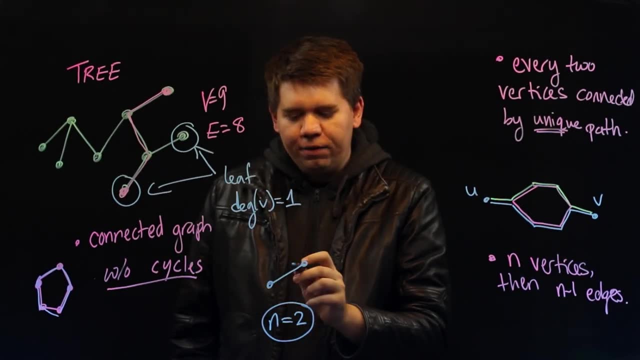 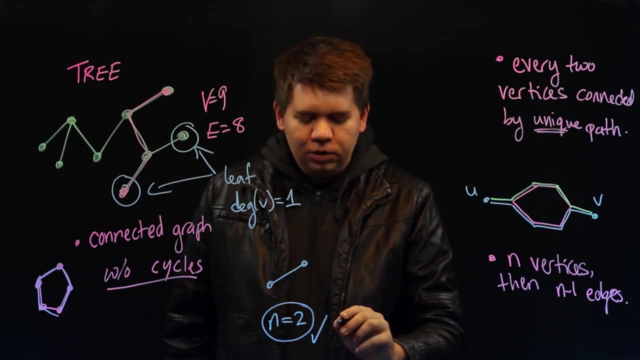 where there are just two vertices in your tree, Then they'll have to be connected by an edge in order to make sure it's a connected graph, And so you'd have two vertices and one edge. Okay, so the fact holds when N equals two. 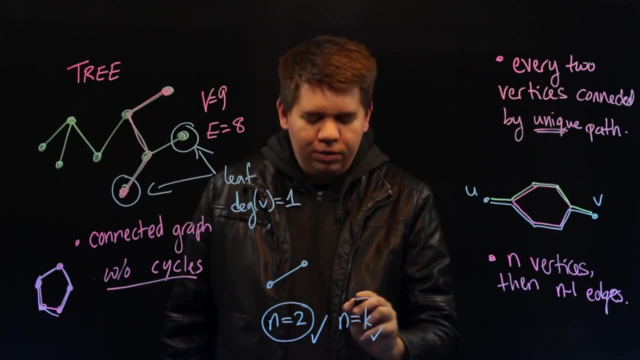 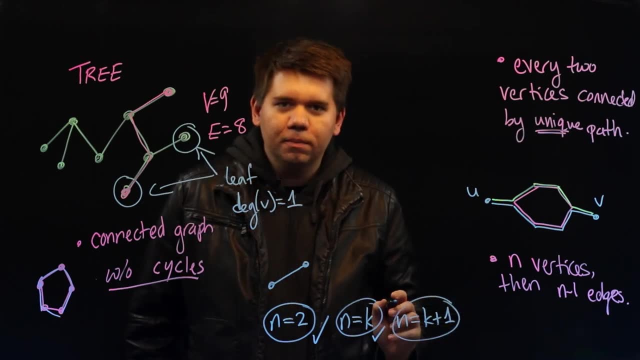 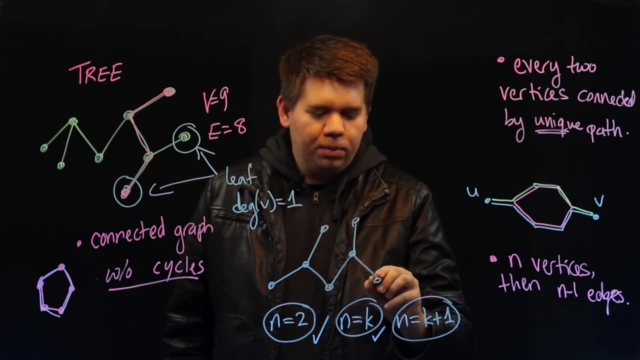 So we're gonna assume it's true when there are K vertices. And now we need to show it's true when there are K plus one vertices. So imagine some graph that has K plus one vertices, A tree with K plus one vertices. We don't know what it looks like. 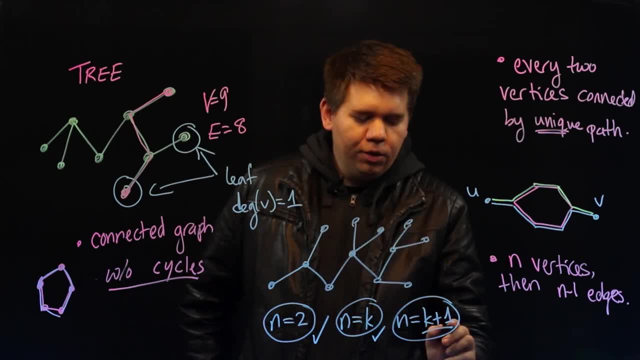 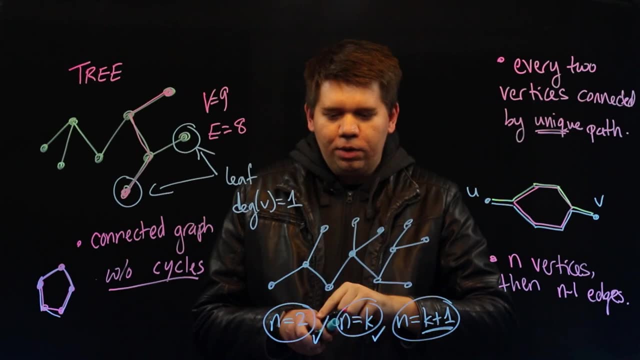 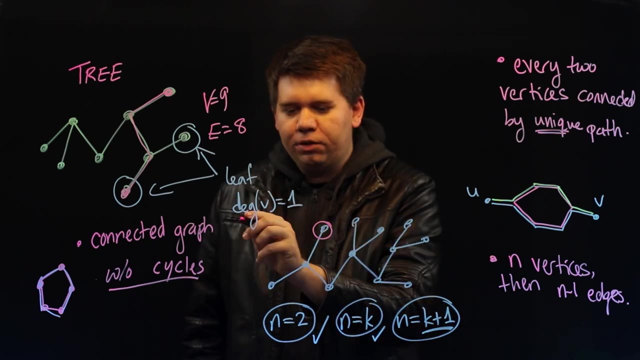 It could look like anything, But you have some tree with K plus one vertices. Well then, since we said every tree has a leaf, you can pick some leaf of the script, This graph, And we know the leaf will have degree one.